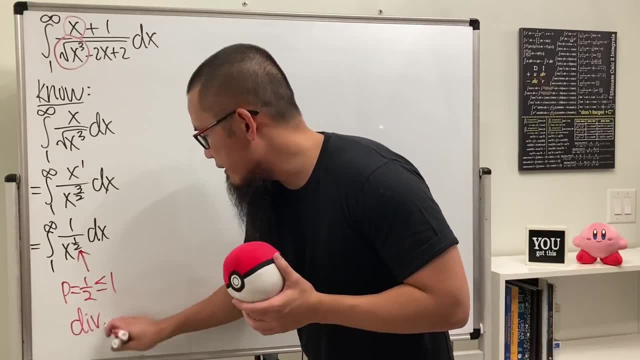 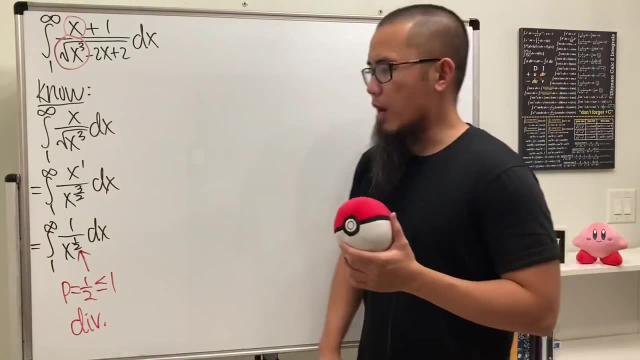 Therefore, we know that And this right here diverges. Okay, So now we have a divergent integral. The next step is that we are going to do the check And I want to put down some notes right here for you guys. first, 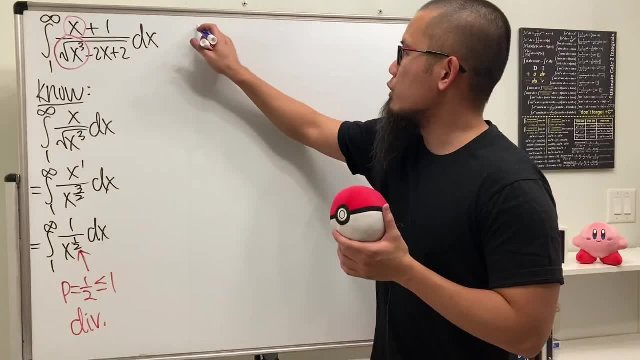 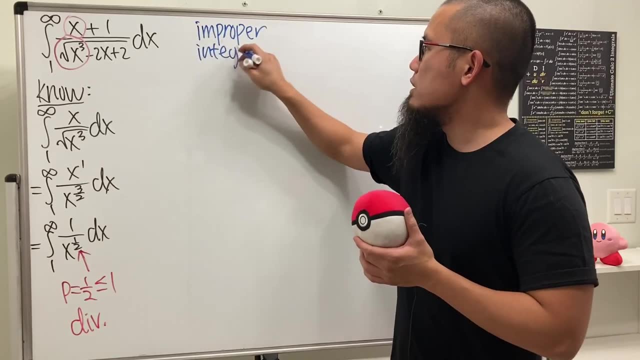 This is the improper integral that we're trying to find out, So let me just go ahead and write that down. If today we have an improper integral that we're trying to find out if it converges or not, But I cannot integrate that. 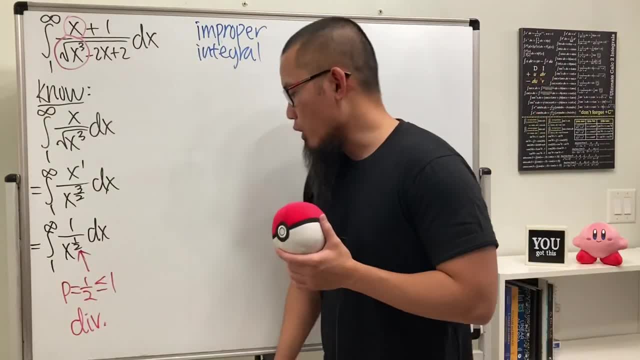 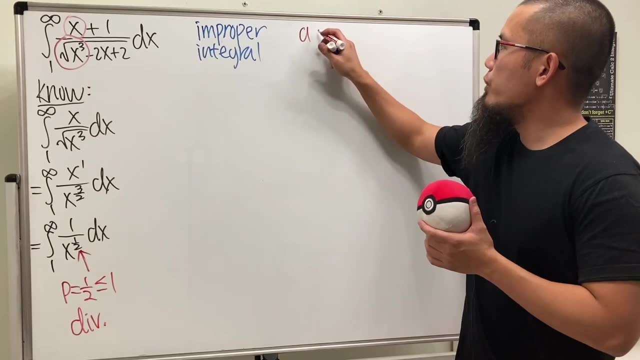 Then use the completion test right, Pick up something that we know much better, which is the one that we have. This right here diverges. So right here, I'm going to write down: okay, we have a non-divergent integral that we are going to work with. 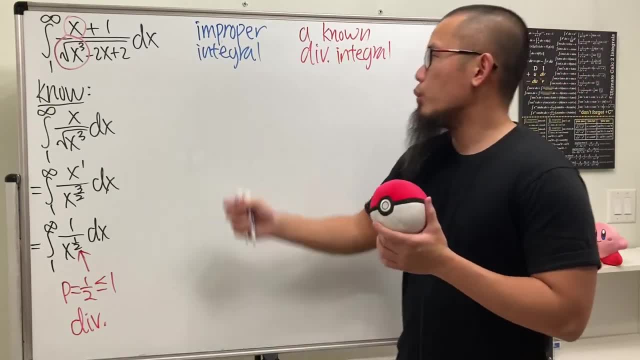 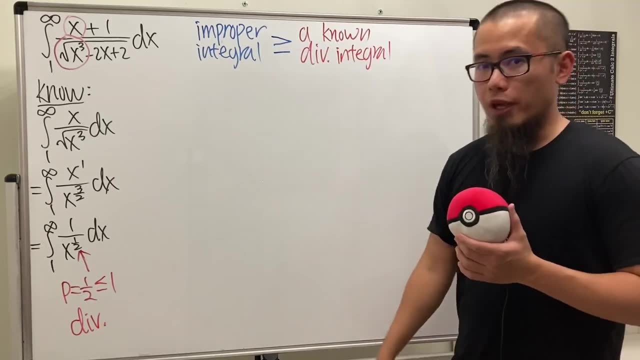 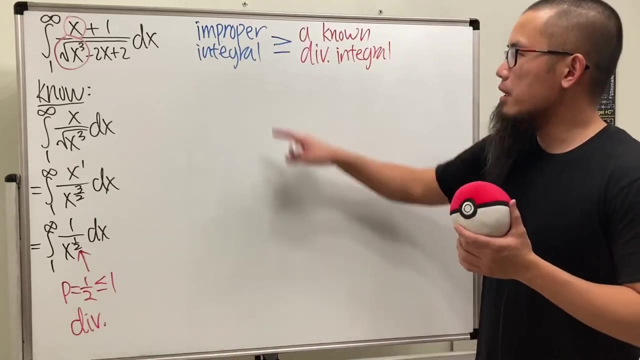 So in this case, what we want to show is: we hope that this improper integral is actually bigger than or equal to the divergent integral right here. Well, this right here actually goes to positive infinity, just like the one over there, Because that way you can see if this right here is bigger than or equal to that. 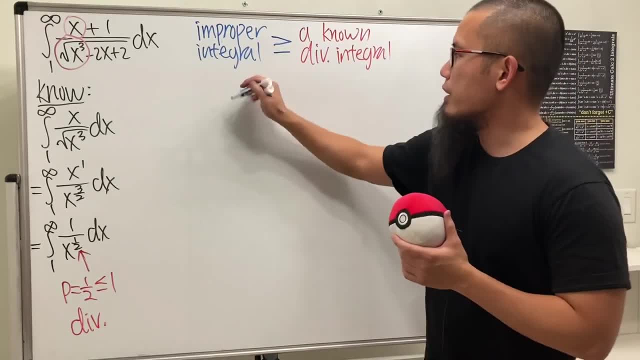 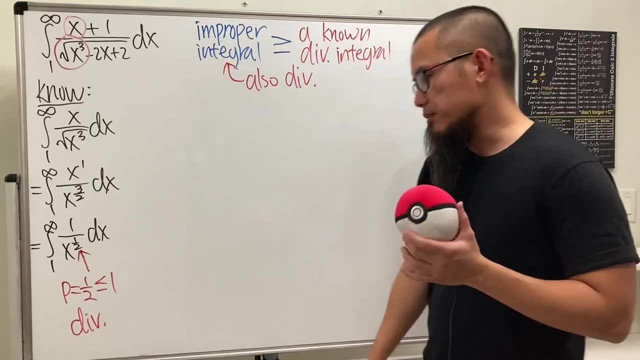 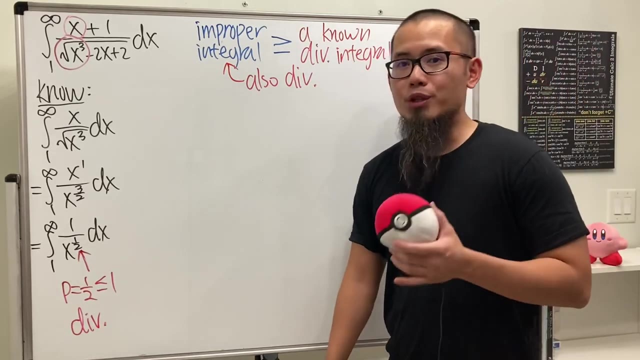 this right here has to be even bigger. Therefore, we can say that this right here also diverges. So that's the idea. But here's a small trouble: What if this divergent integral goes to negative infinity? Well, the best answer I can give you guys is that we don't want that. 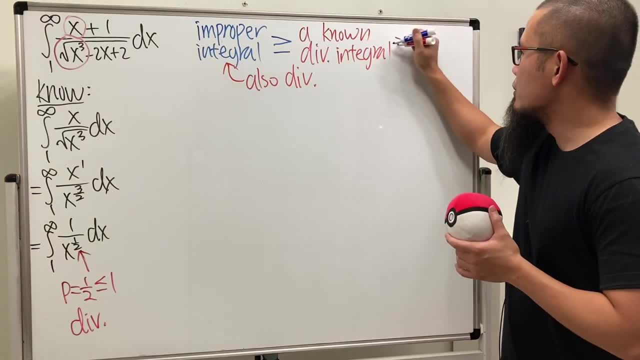 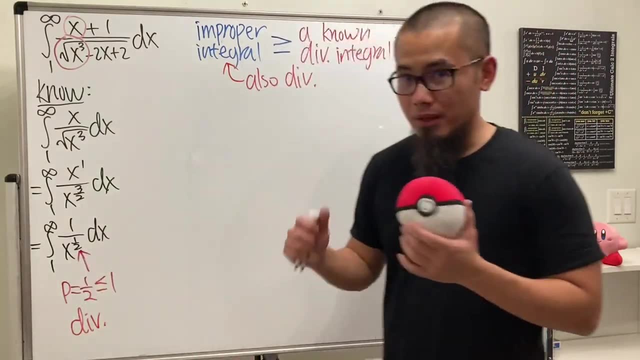 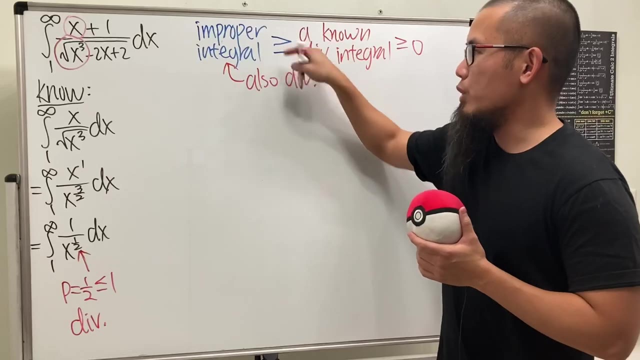 So, to take up that situation, just make sure that everything is positive so that you don't talk about the negative infinity case. This right here thus diverges to positive infinity, So we can definitely use that And again, this is the inequality that we hope to show. 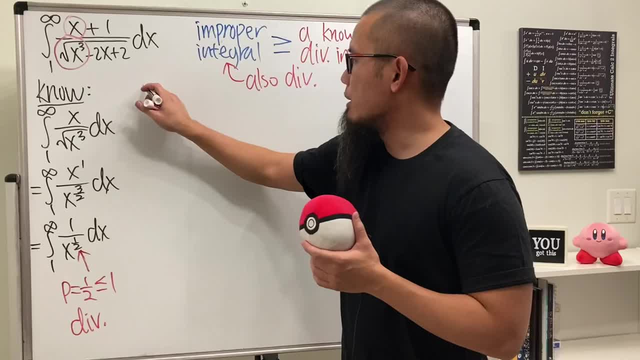 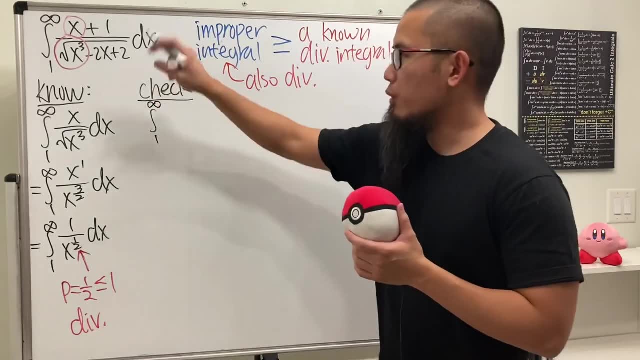 Now we just have to go ahead and do the check. So let's go ahead and put that down right here real quick. Put down the one that we are trying to do, which is the integral from 1 to infinity of all that. 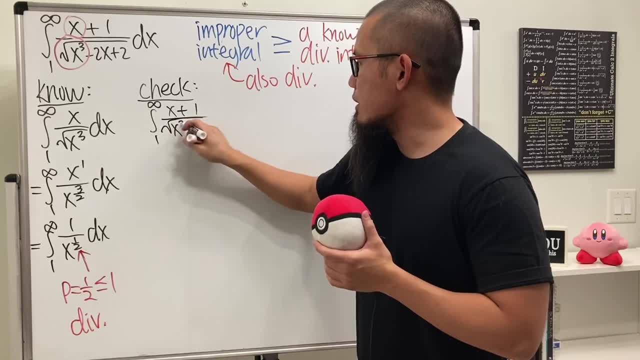 x plus 1 over square root of x to the 3rd power. So that's the integral from 1 to infinity of all that x plus 1 over square root of x to the 3rd power. So that's the integral from 1 to infinity of all that, x plus 1 over square root of x to the 3rd power. 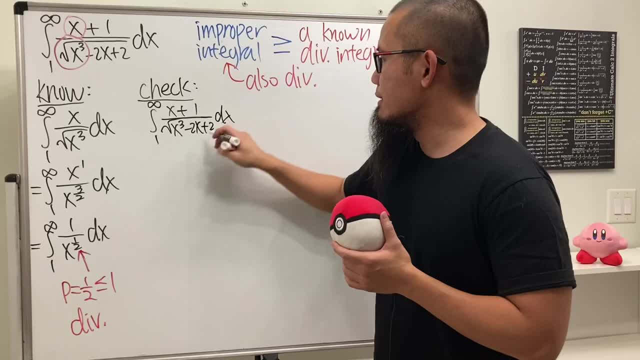 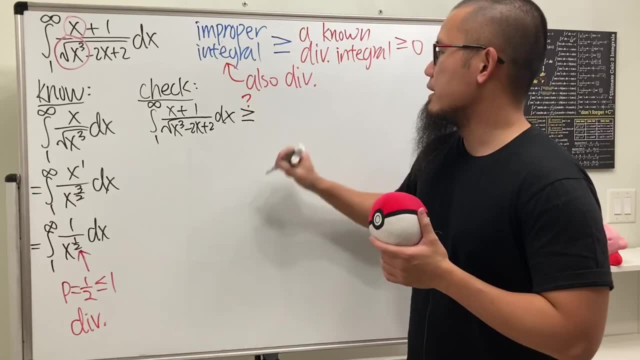 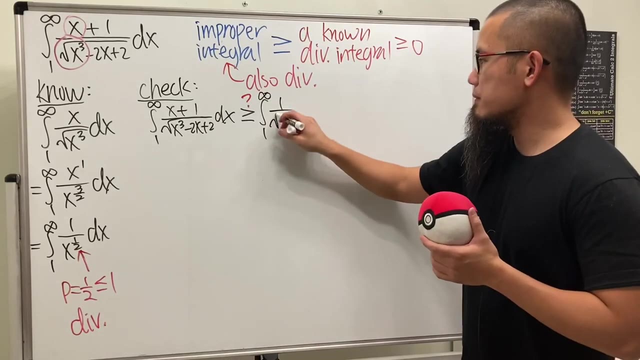 power minus 2x plus 2 dx, and then, by what we said earlier, we hope to show that this is bigger than we're equal to, but we don't know yet, and then we want to put that down. we hope that this right here is true, and let me write that as the square root of x. all right, keep in mind this inequality is. 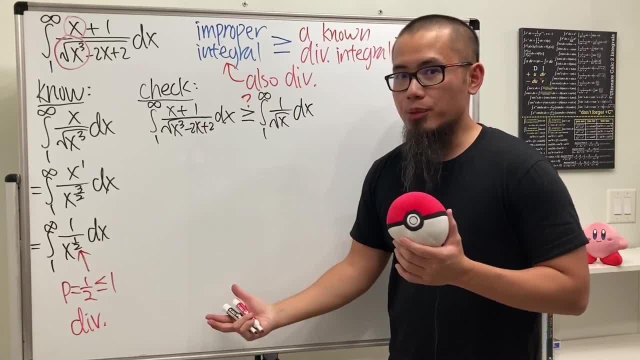 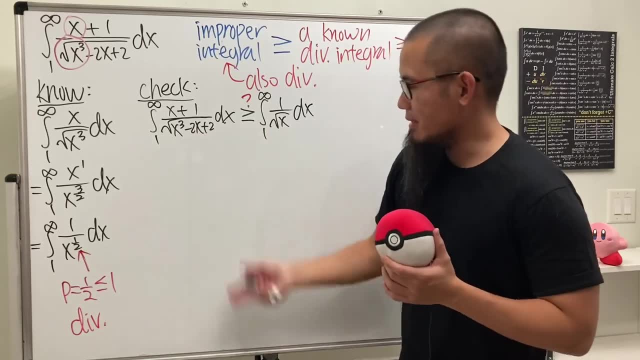 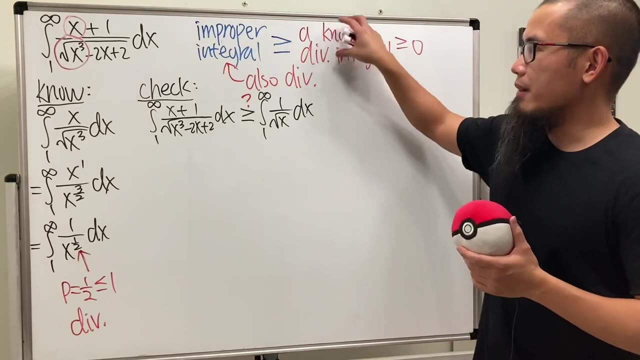 extremely crucial and if the work ends up to be good, that means if this right here is actually true, then we can draw conclusion. if this inequality is not true, then we cannot draw conclusion. that means we may have to try something else and imagine: if you have a diet, if you have a conversion. 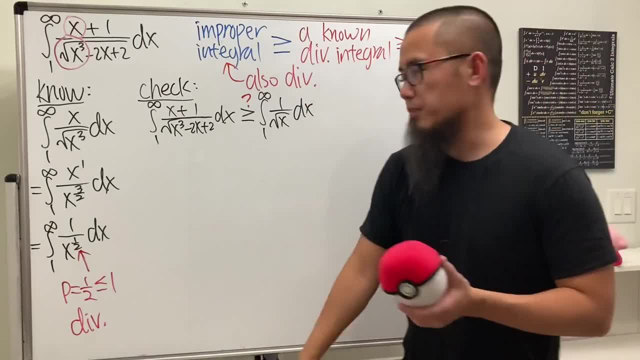 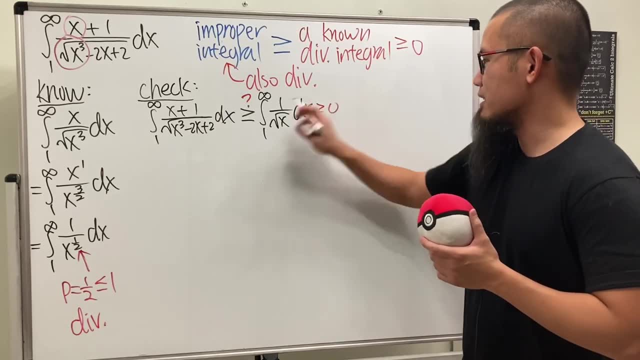 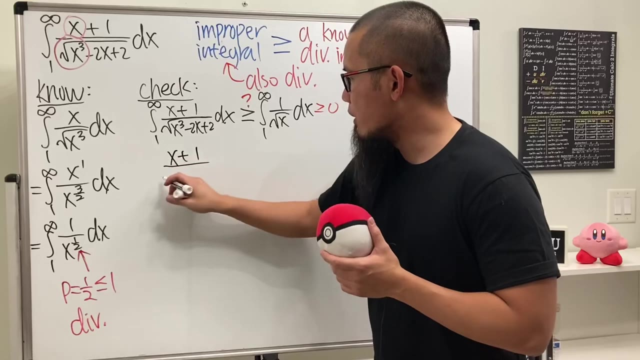 integral. here you actually switch that wrong, which is the next example. all right, so just wait for that, but anyway, let's take care of this first. first off, notice that this is positive, so everything's positive. don't worry, we can then just compare the inside. so right here, let's look at x plus one over. 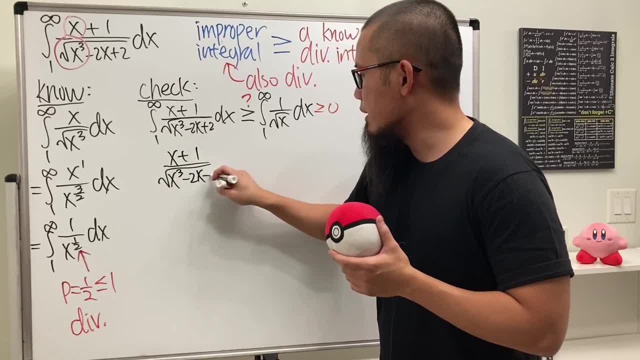 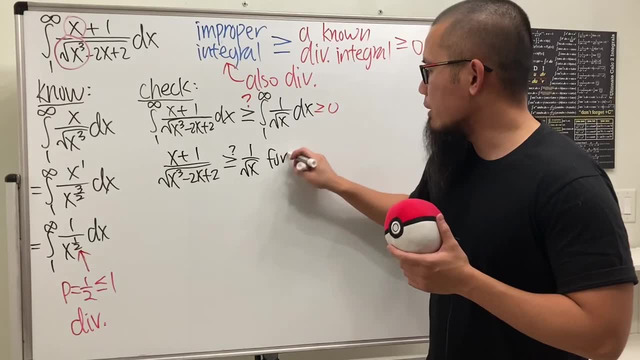 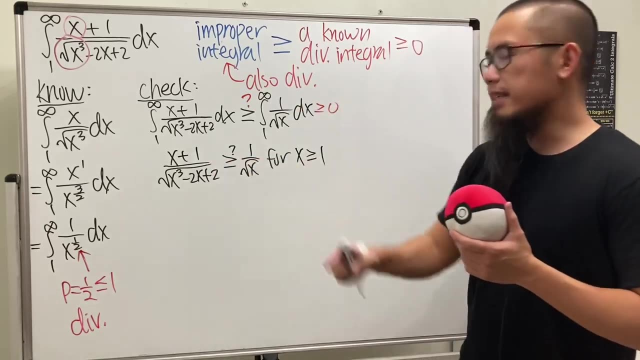 square root root of x to the third power minus two. x plus two, and again we hope to show that this is greater than or equal to one over square root of x, and we just care about when x is one or bigger. so we can say x is greater than equal to one, and then this is nice to see, but it's okay because we can just 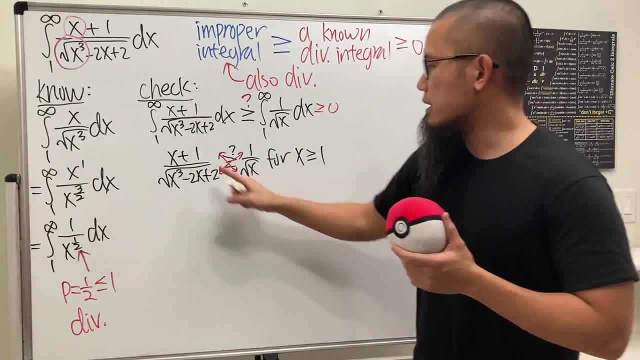 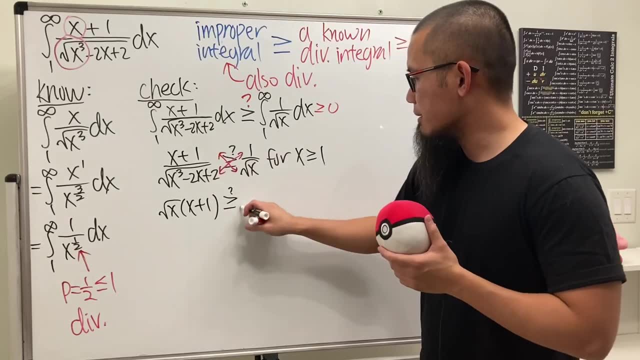 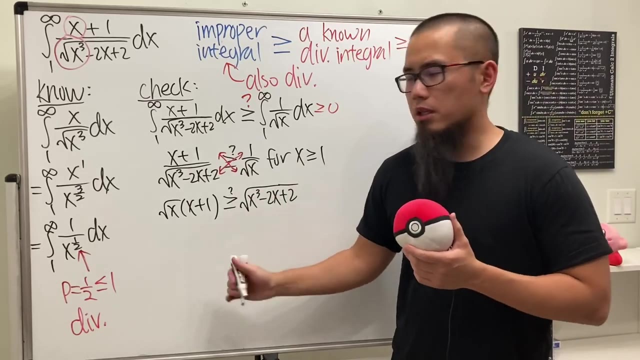 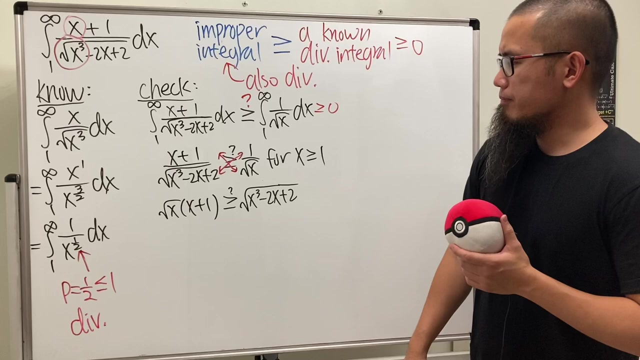 cross multiply and you see this times that is going to be square root of x, times x plus one. is this greater than or equal to that? times that? and notice, i kept the same inequality because everything's positive, so i can just cross multiply without any worry. and now, hmm, what do we do with this? well, you have a couple ways to do this. 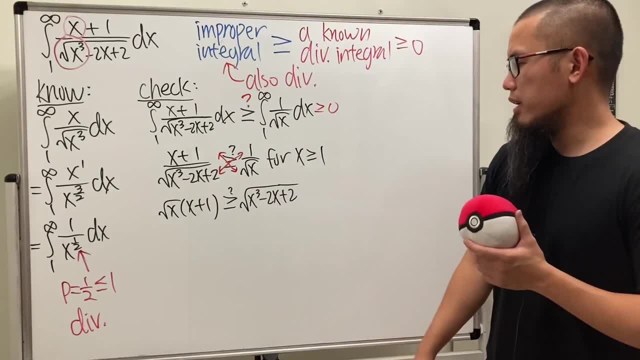 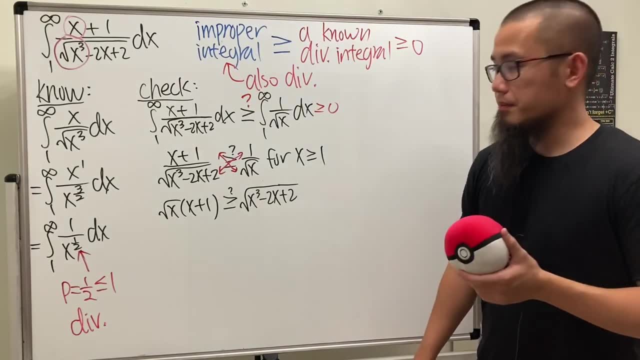 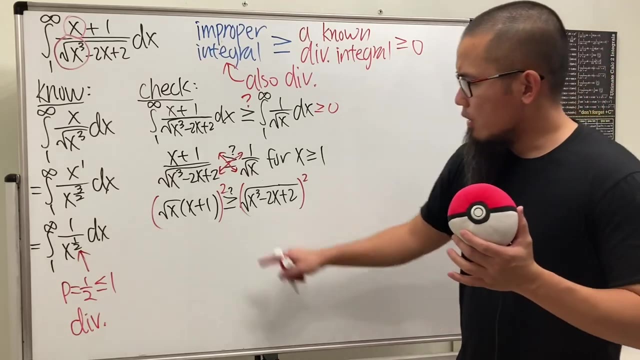 you might want to just distribute that inside, that's totally okay, and then draw some comparison and um. or if you want to get rid of the square roots, you can square both sides here. let's go ahead and do the second one, which is square both sides. but when you square both sides, 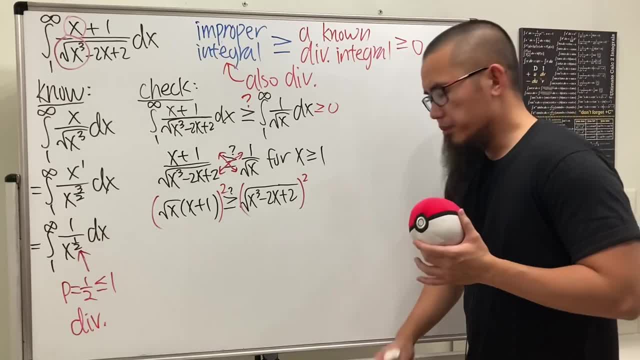 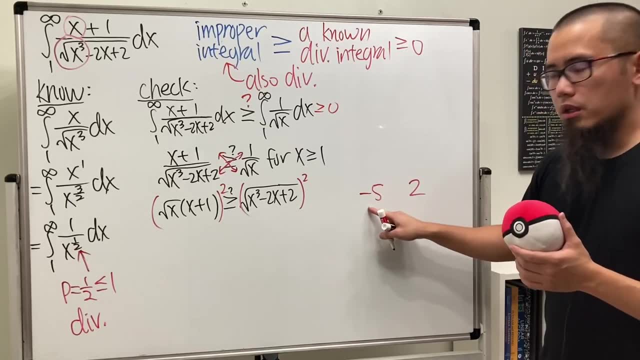 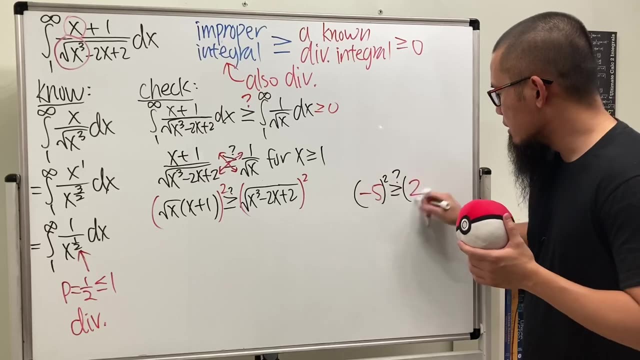 you have to be really, really careful, because you see, if you have negative five versus two, is this true? this is not true? right, of course not. but if you square both sides, guess what? we end up with positive 25, and then this right here is four, and it becomes true. 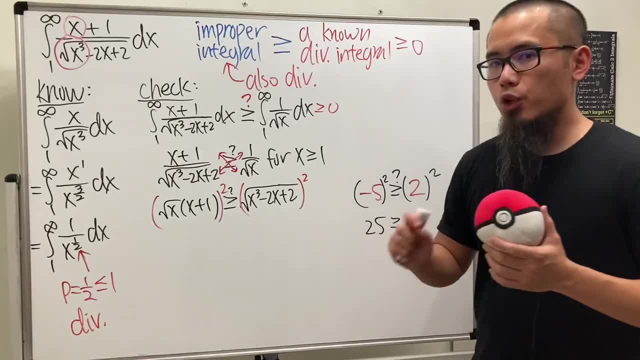 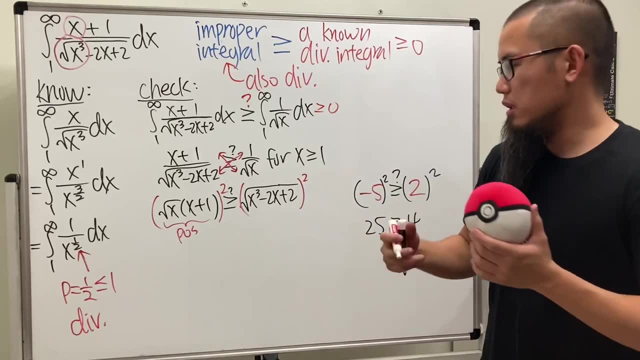 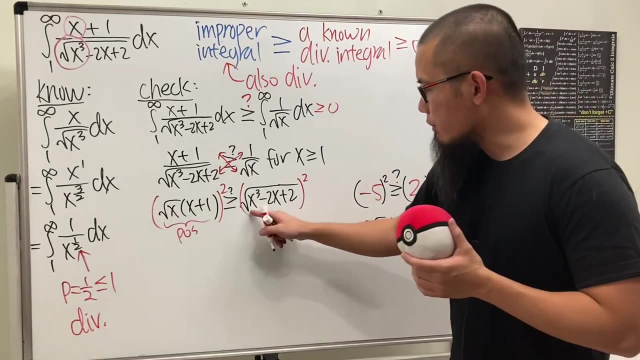 we don't want that to happen. when you square both sides, you will have to make sure that the inside is positive. this is the reason why that we have to really care about if an expression is always positive or not. this is indeed always positive on this interval. likewise for this one. 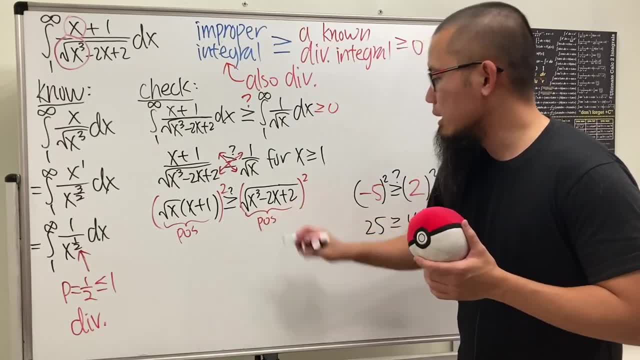 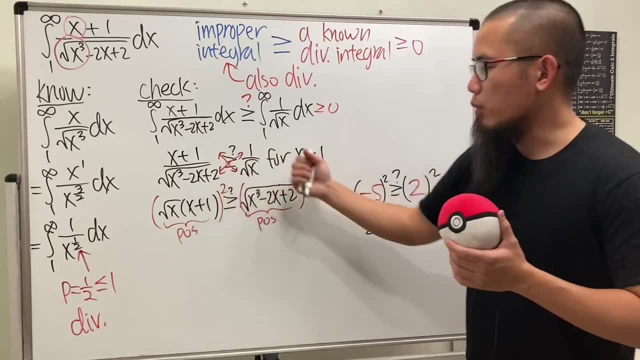 right here. it's also always positive. if you have a positive number, it's greater than or equal to a positive number. you can still square both sides and you can make sure that the inside maintain the same equality. but if you have a negative and then a positive, if you compute that, 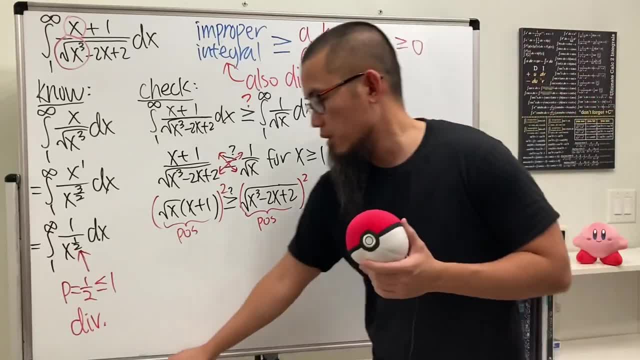 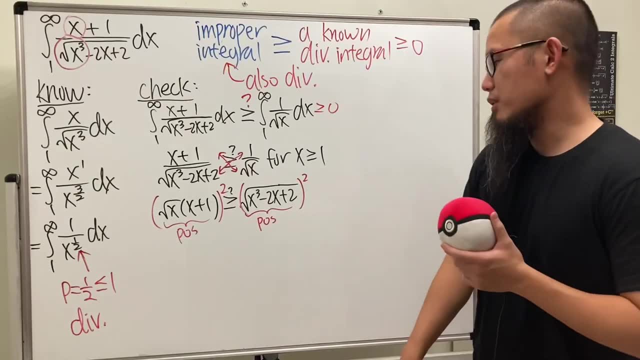 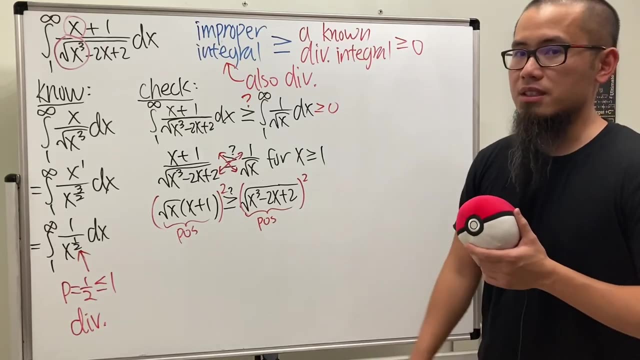 after you square both sides, you know the inequality might be switched and all that stuff. so yeah, so just indicate that you are, that these are the technical details. that's so, and why is this positive? you can do the graph of this real quick and you will see that this is indeed positive. 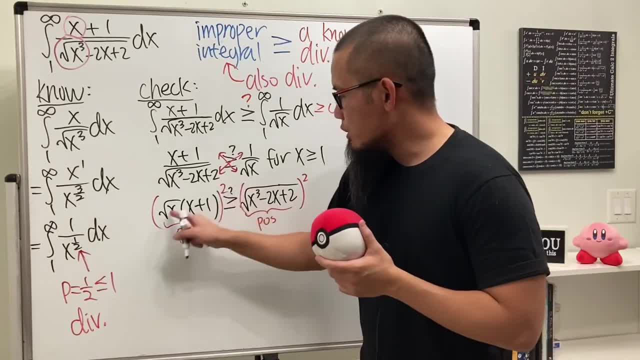 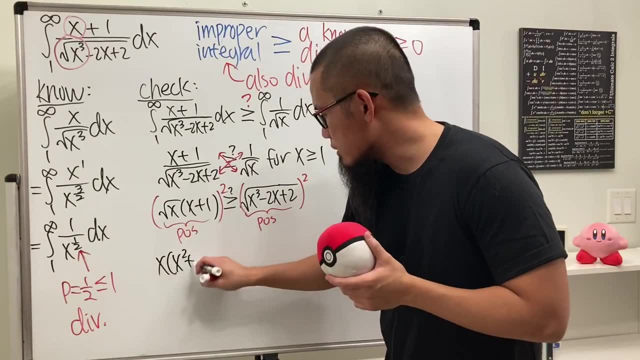 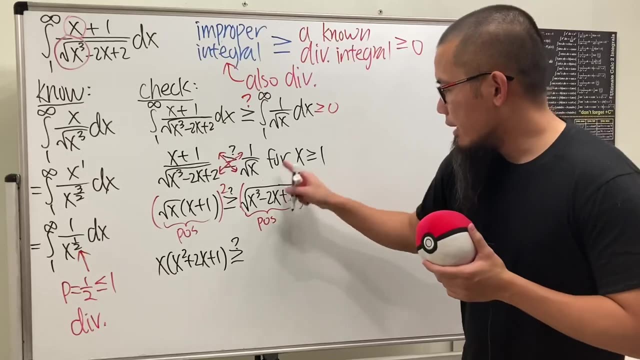 all right. so now let's see when we square this, this becomes just x, and then x plus 1 square, which is just x square plus 2x plus 1. is this greater than or equal to? you see, we kept the same inequality and square square root cancel. so we just get the x to the third power minus 2x. 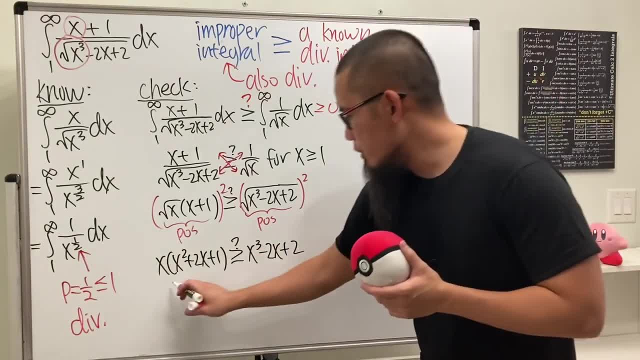 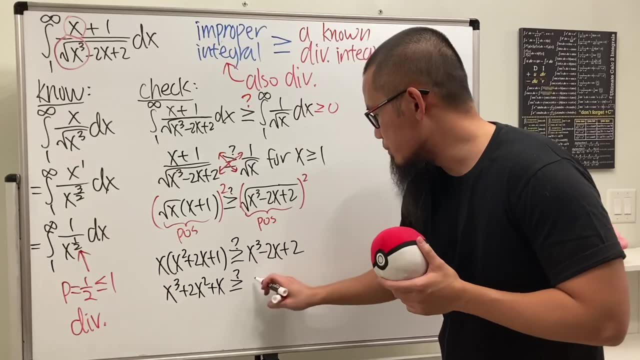 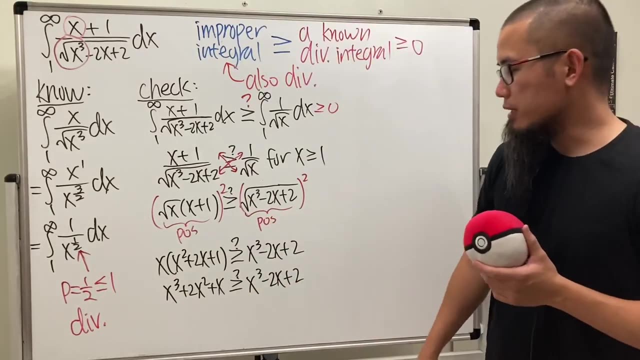 plus 2, and of course we can distribute. we just get x to the third power plus 2x square, and then plus x, and then is this greater than or equal to this expression? well, we can get rid of the x to the third power on both sides and we can move this to the other side. 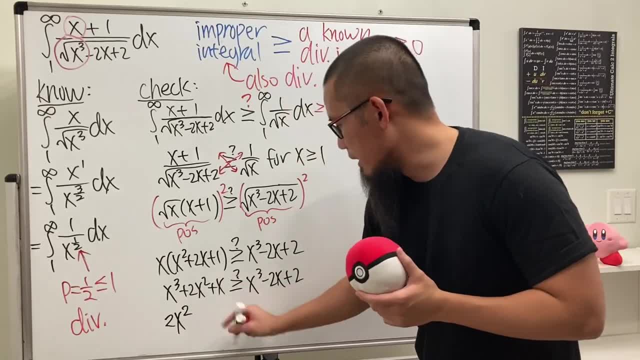 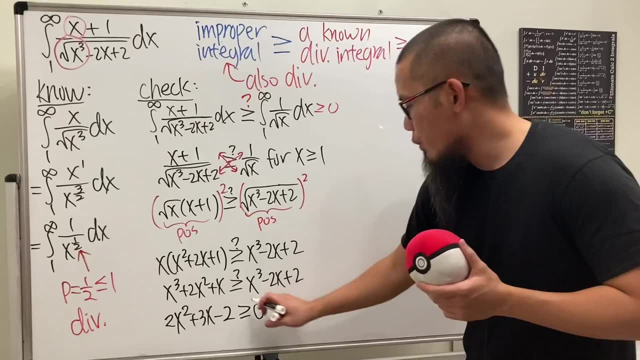 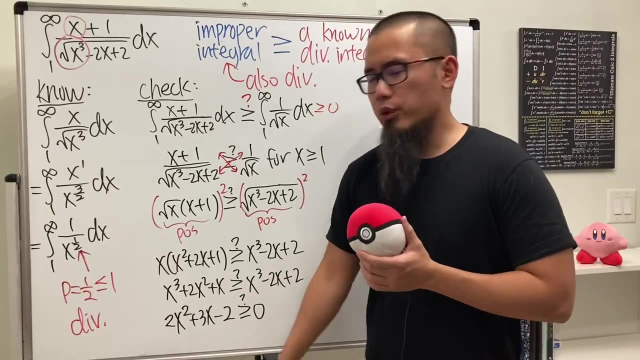 so we get 2x square plus 3x and then minus 2. is this greater than or equal to 0? well, we do have a minus right here, so we have to be careful. one way to do this right here is that you can just: 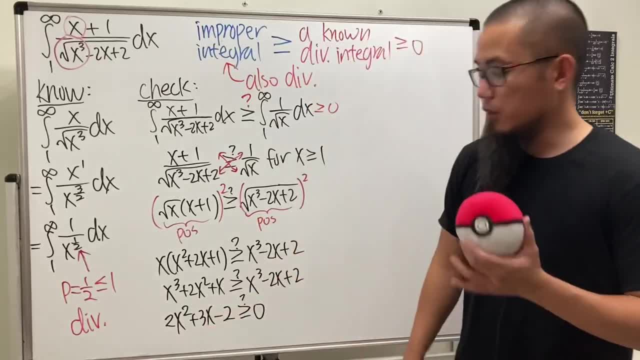 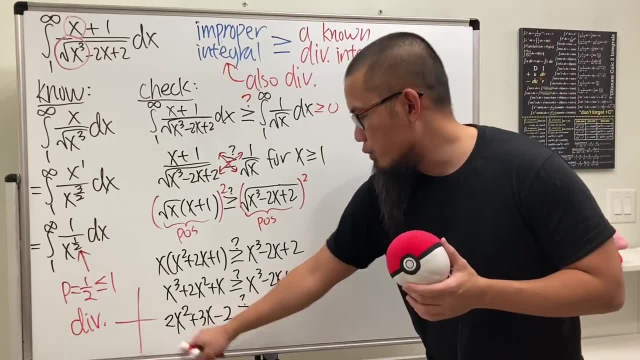 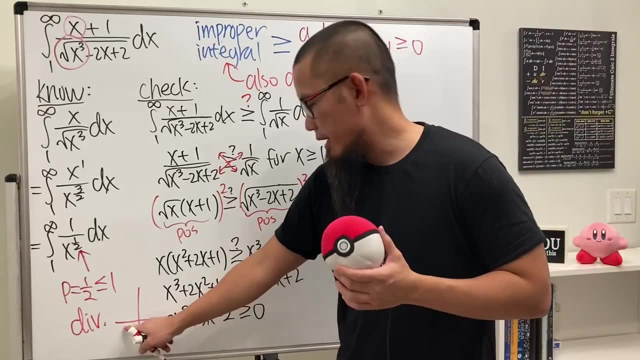 okay, the vertex is that negative b over 2a, which is going to be negative 3 over 2 times 2, so it's negative 3 over 4 is going to be somewhere here and then you plug in and you will get a negative. 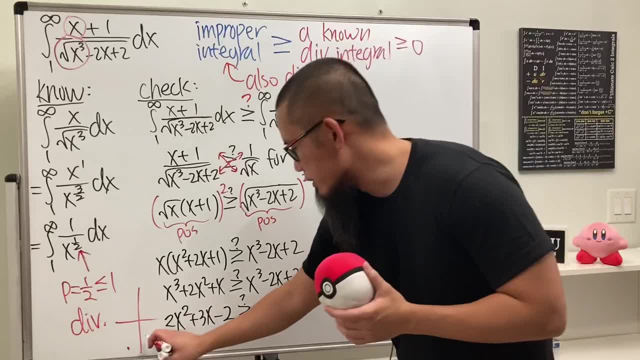 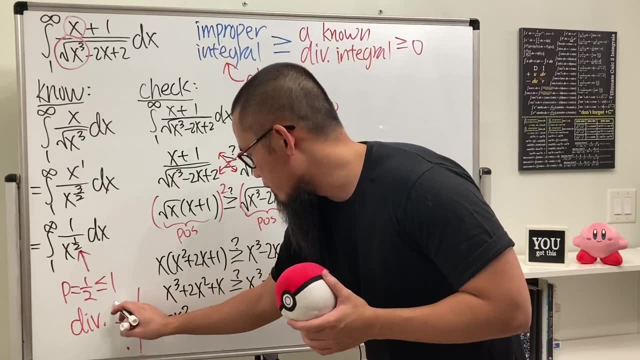 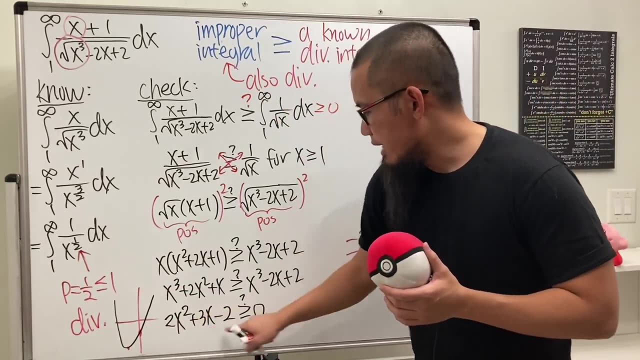 value right, and when x is equal to 0, you will see that it's a negative 2 right, and you can pretty much see the graph will go like this. so i'll just go ahead and draw it real quick: when x is 1, put it here this and that will cancel. we just get 3, so you know. 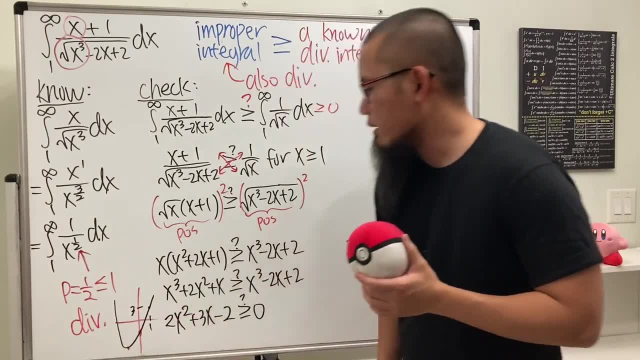 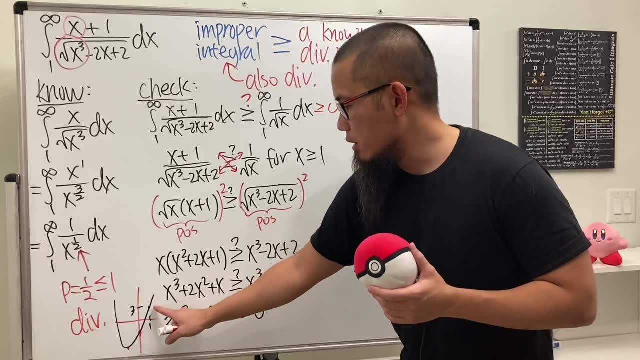 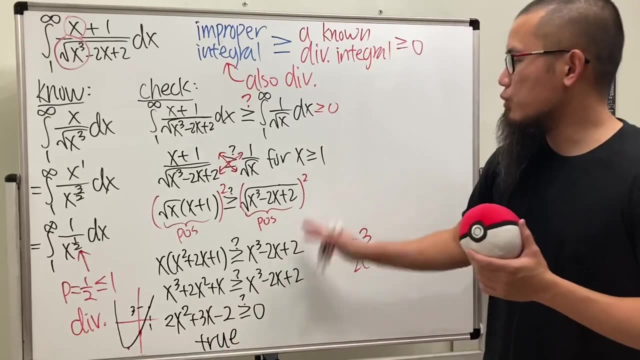 this right here will be 3, right 1 and 3. so now with that graph you can see that this portion, when x is bigger than or equal to 1, it has to be greater than 0. so this right here is definitely true. right, it's true for x is greater than or equal to 1. 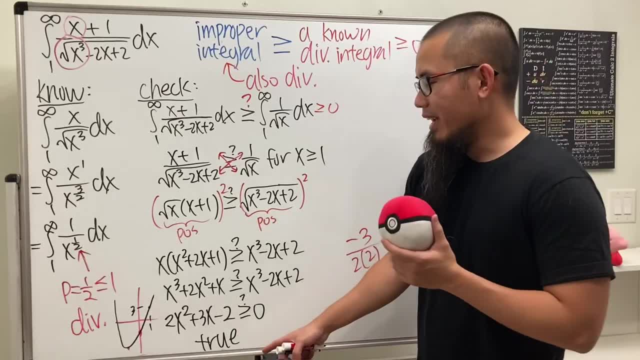 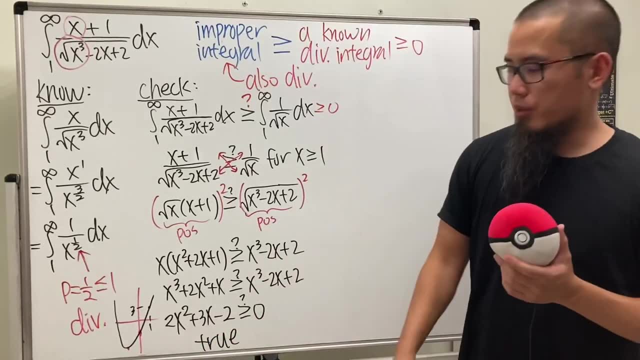 because i needed this to be true and i just put down true without doing any convincing work. i will have to provide a graph to make sure that that is indeed true and do not just plug in a number, like sometimes. if you plug in number it might not work. you actually have to do a legitimate. 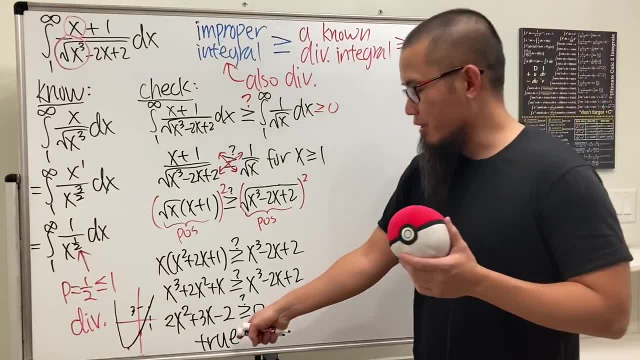 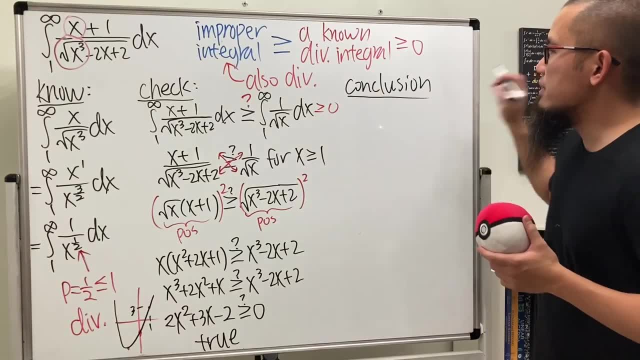 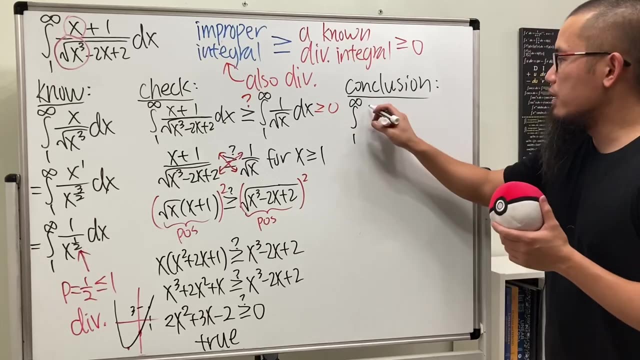 reason for that? yay, we have a true statement right here, so that means we can go to the next step, and that's going to be the conclusion. perfect, so, for the conclusion is that we're just going to state what exactly is up with that: the integral going from 1 to infinity of x plus 1 over square root of x. 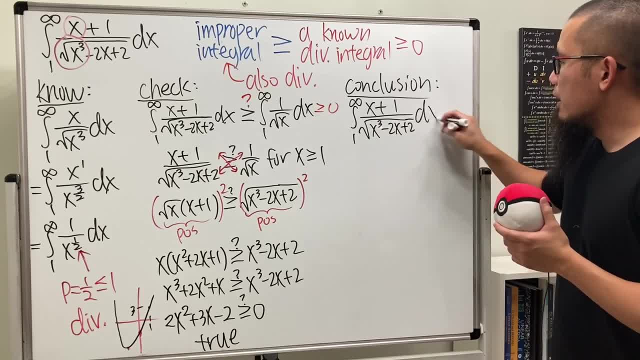 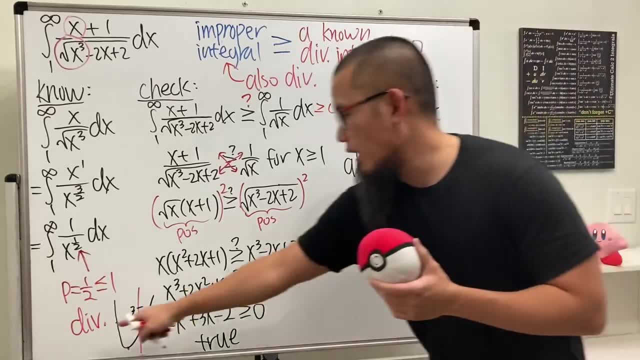 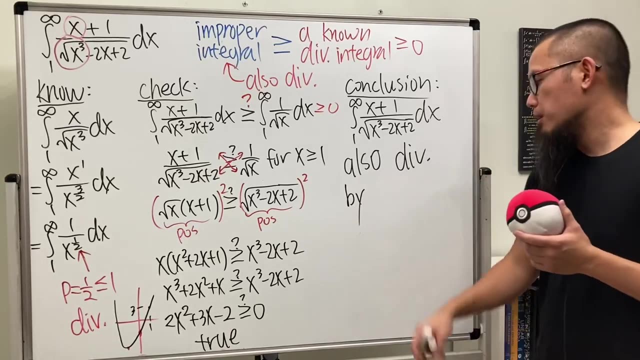 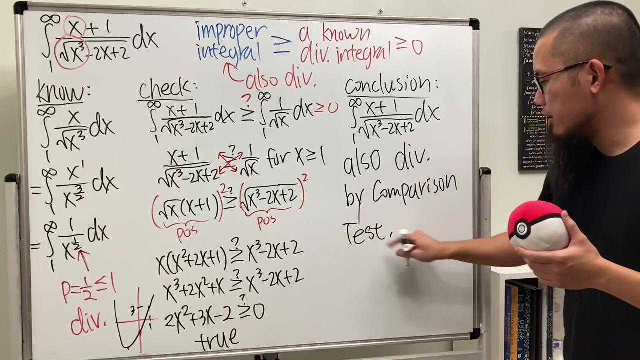 third, power minus 2x plus 2.. this right here, let's use the word also also what also diverge, just like the one that we know also diverges and we can provide a nice reason by the comparison test. so this, right here, is how you write the three steps: proof for the comparison test put down. 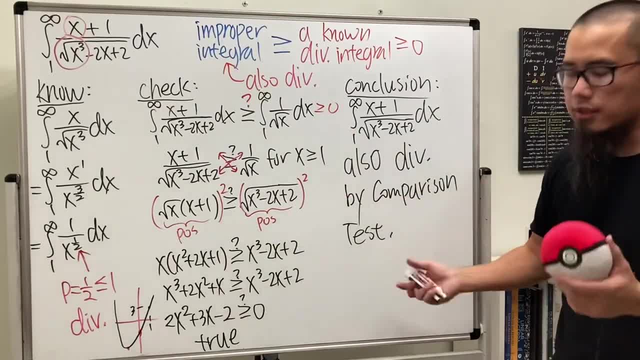 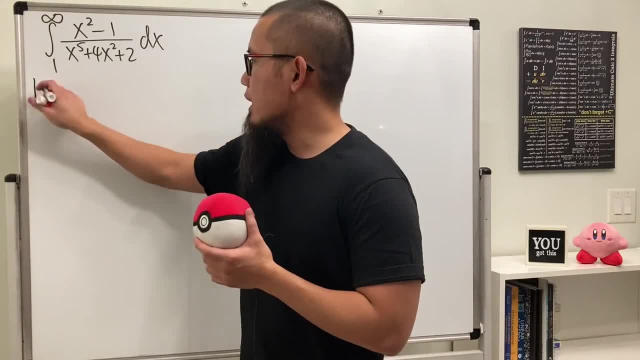 what you know, do the check and then draw the conclusion. then this right here shall be really, really clear. here is the second example, and of course, we are going to do the same three steps. so let's begin with putting down what we know, and that's just going to be the highest power. 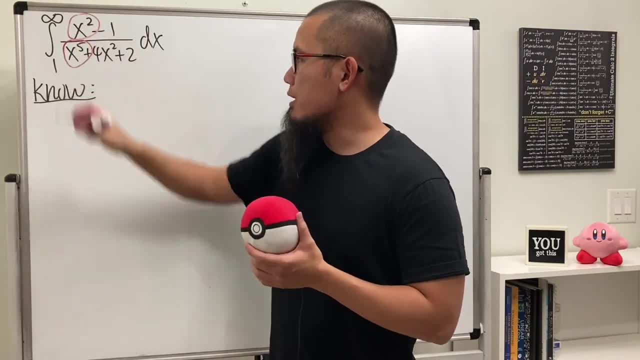 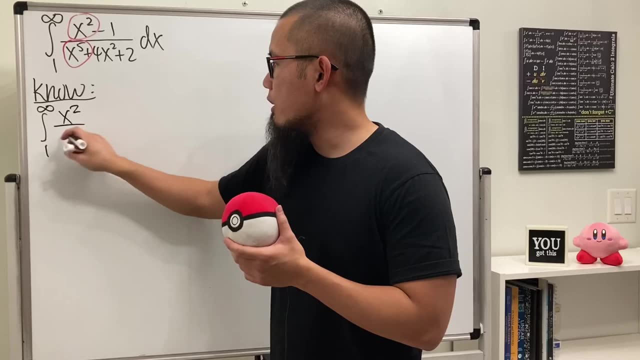 of x on the top, which is this, and then the highest power of x on the bottom right. they are the dominating parts. so we are looking at the integral going from 1 to infinity, and we have x squared over x to the fifth power, and we can reduce this and we just get integral. 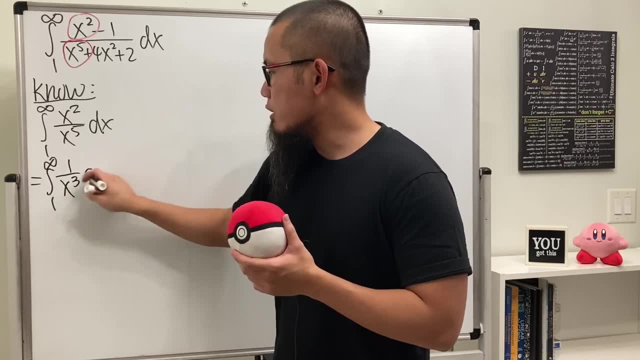 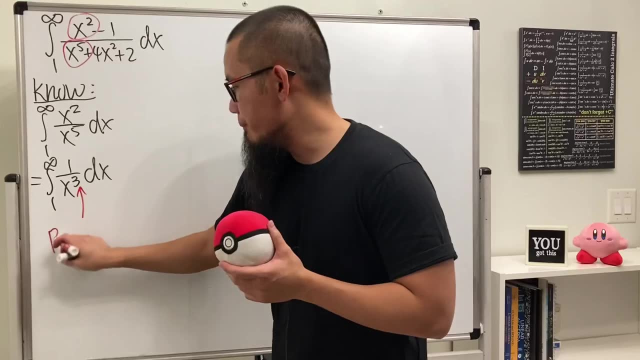 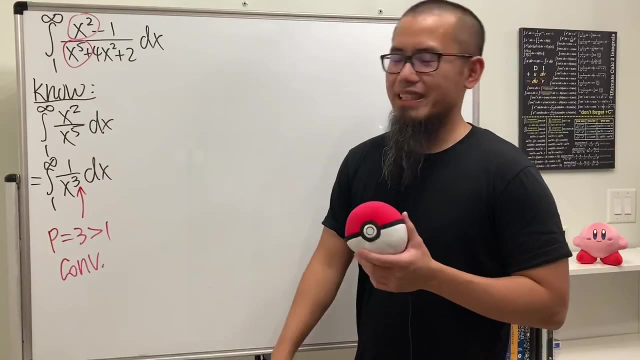 going from 1 to infinity of 1 over x to the third power. and this is so nice because this is once again a p integral. p is equal to 3, which is greater than 1. therefore, we know that this, right here, converges. so now let me put down the notes for you guys. when we have a convergent integral to: 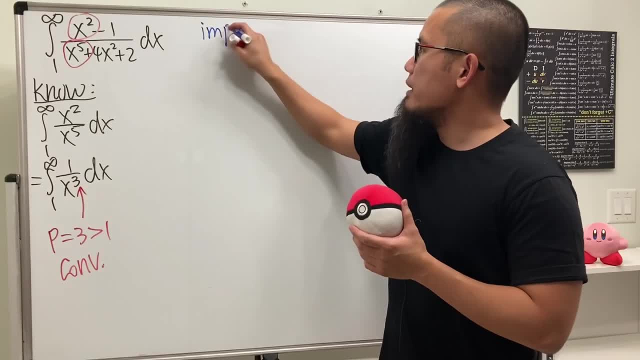 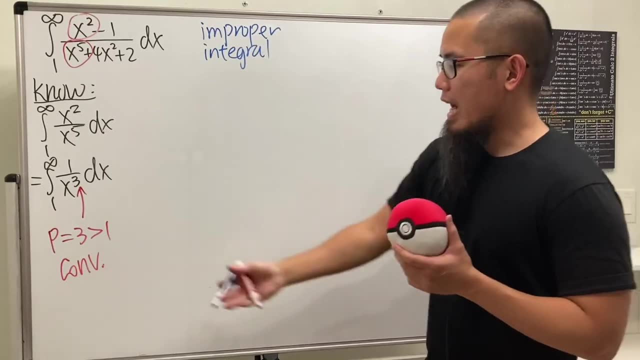 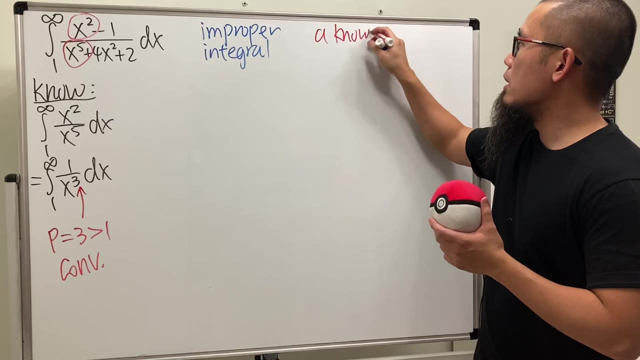 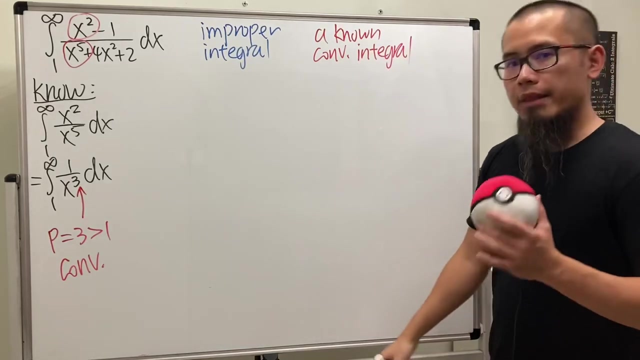 that we know. so, right here we have an improper integral that we are trying to find out if it converges or not, and then we have an integral that we know converges. so i will just put down a known convergent integral. so we already know this right, and now this is what we want to show. 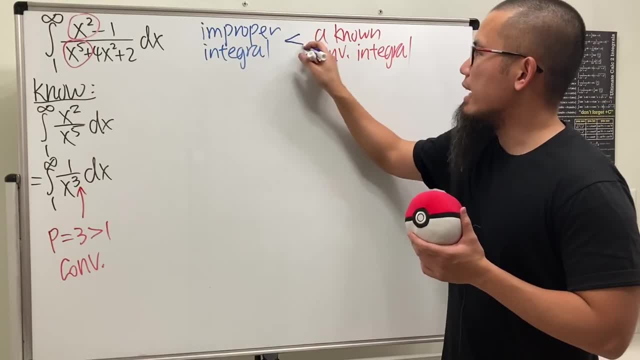 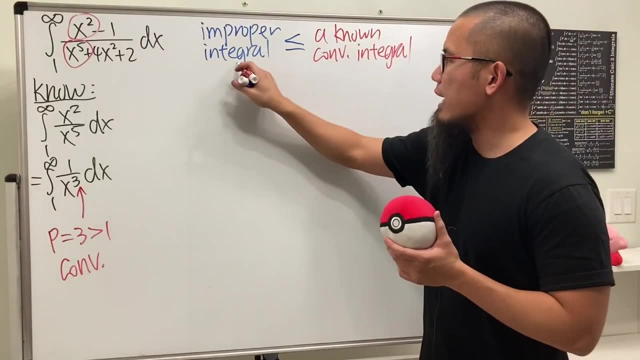 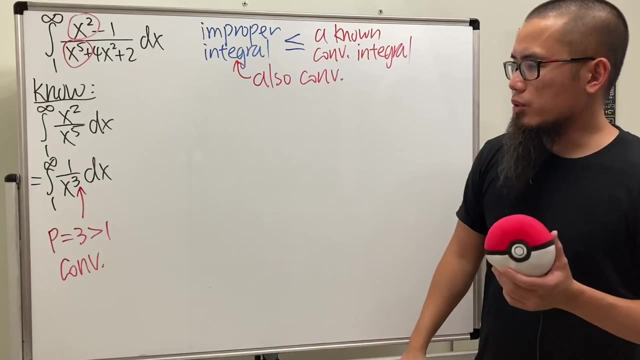 we hope to show that this right here is less than or equal to a known convergent integral, because if we can do that, then we can draw a conclusion that this right here also converges. well, why is this true? let's just talk about it: this right here a known convergent integral. 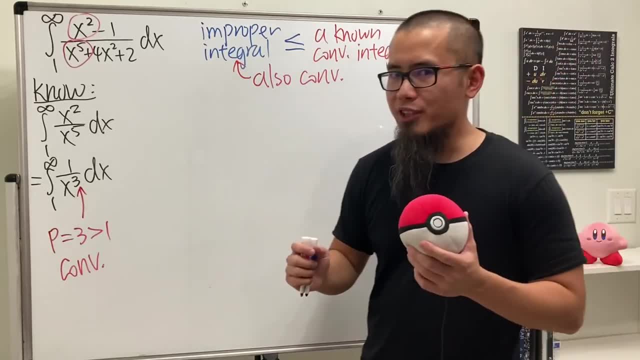 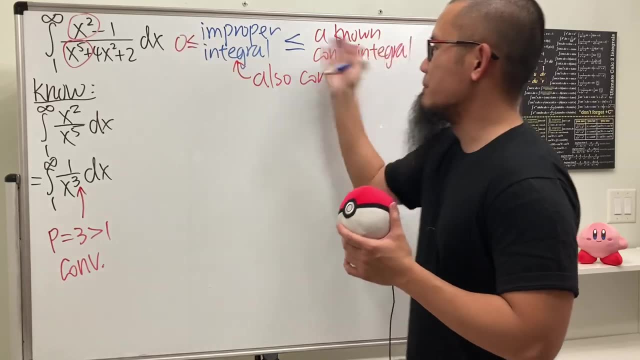 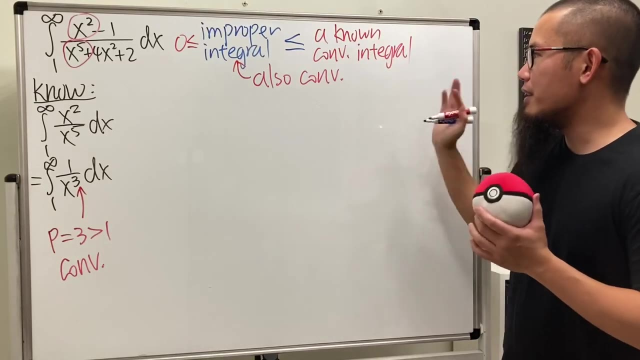 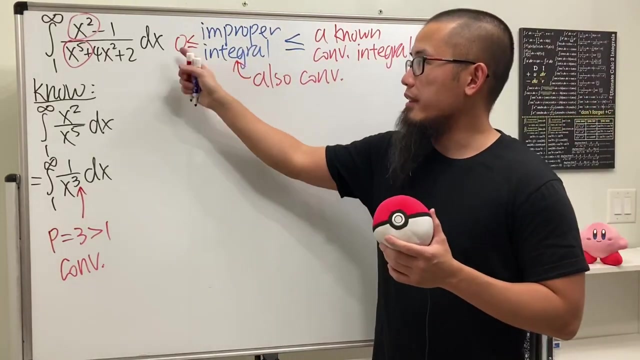 will give you a finite value and of course i should be mentioning positive finite value, so we will also have to make sure that everything is positive. so we are looking at the inequality. so this right here: suppose we do get a positive finite value if this right here is smaller than or equal to a positive finite value, and this right here cannot. 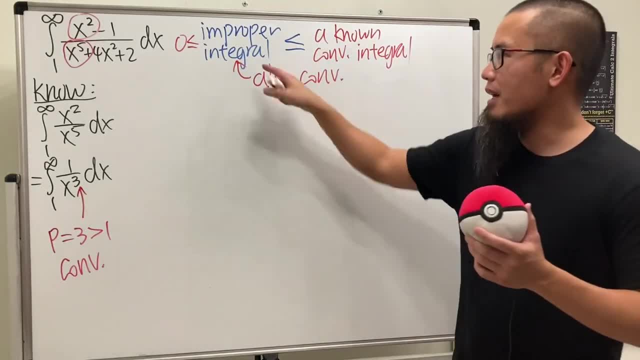 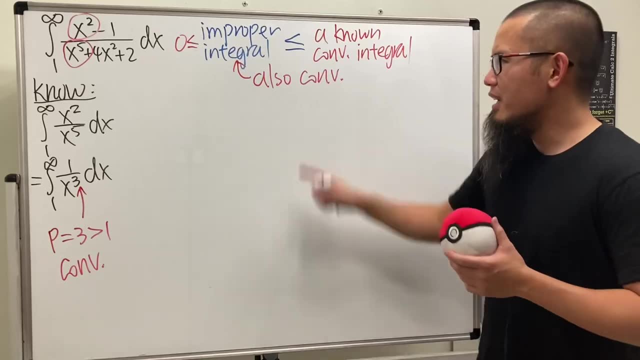 go to negative because we have this right here, then we know that this right here has to be finite as well. it's a smaller finite value, therefore this right here also converges. so this is the inequality that we will have to set up, and we hope that it actually is true so that we we can draw a conclusion. 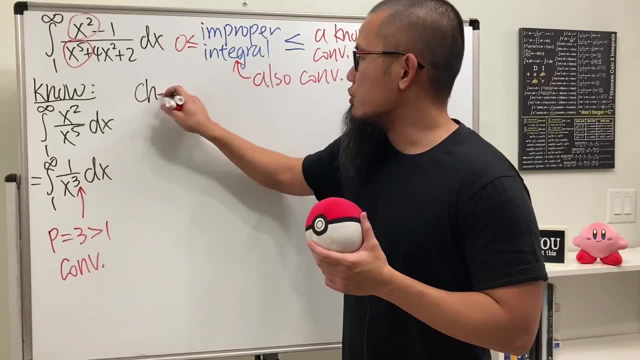 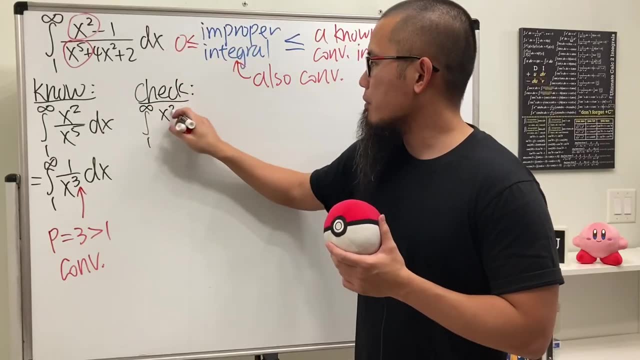 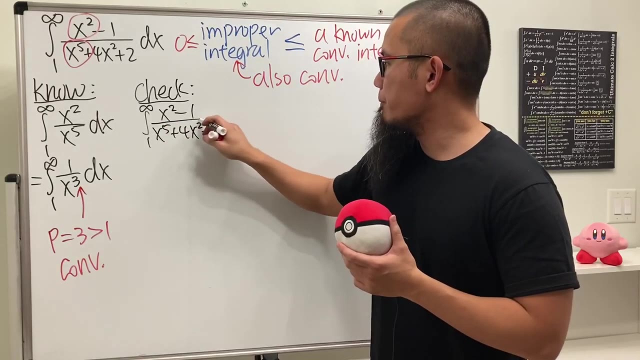 so that we, we can draw a conclusion. okay. so, ladies and gentlemen, here is the check. let's go ahead and put down the one that we're doing, which is the integral one to infinity, and then x squared minus one over x to the fifth, plus four, x squared and then plus two, and then the dx. we hope to show that this, right here, is less. 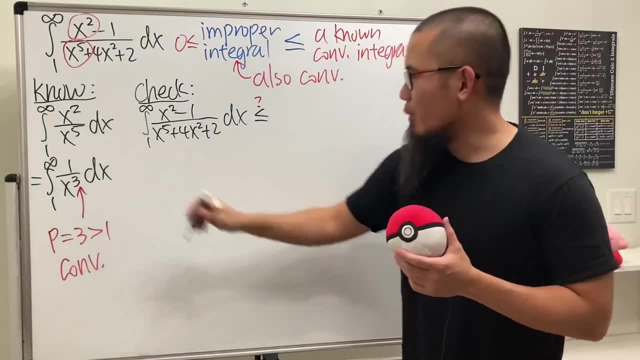 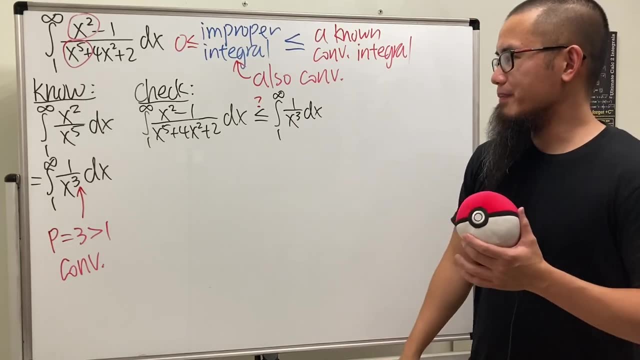 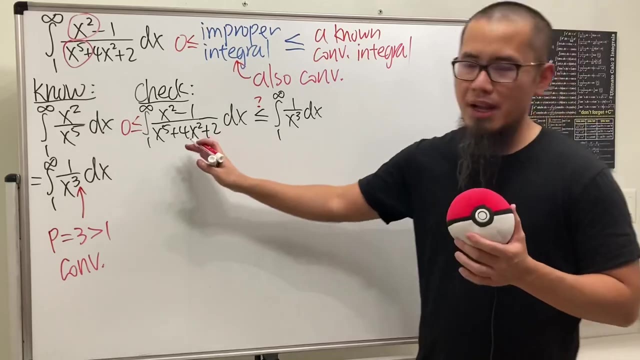 than or equal to, but we don't know yet that one integral from one to infinity of one over x, plus third power, dx. and again, i can promise you guys for this kind of question you can almost always put this down like i will not ask you guys tricky questions. yeah, and hopefully, if you are taking a calculus, 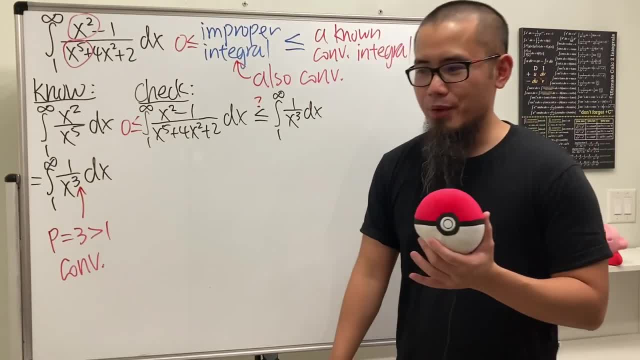 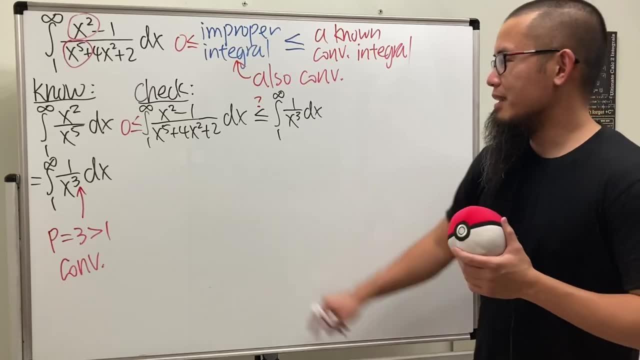 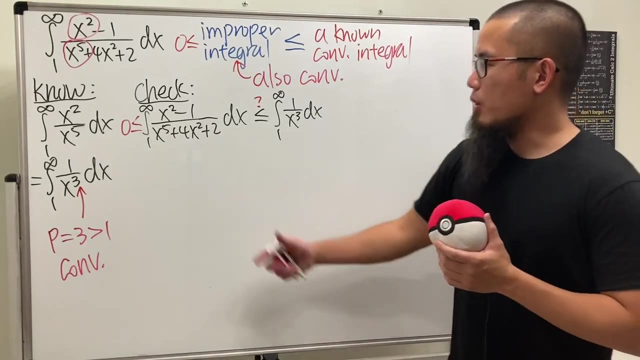 tool from other professors. your, your professor will ask you like tricky questions too, because this right here can get really technical. so yeah, we don't want that yet, but anyway, at least for my videos, when for my examples you can do that. but yeah, all right, so same business. 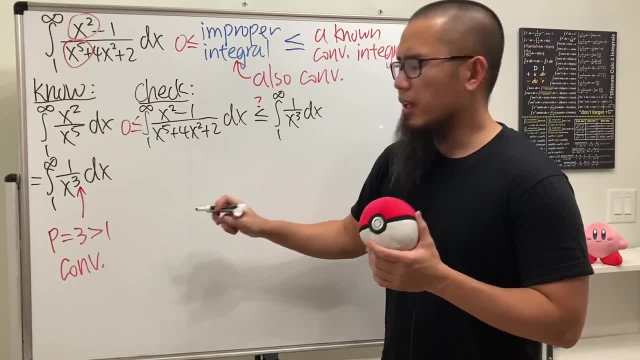 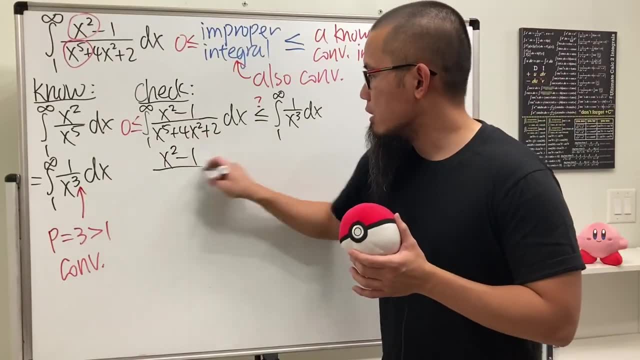 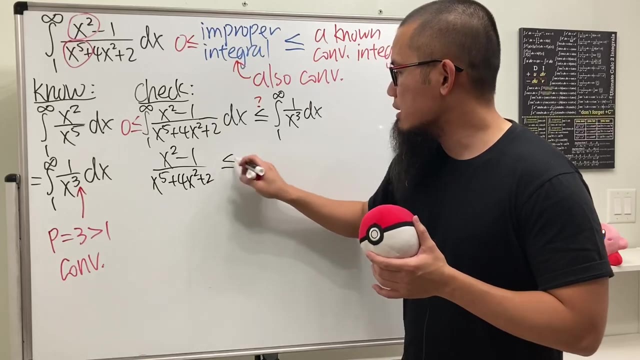 as what we did earlier, we're just going to compare the functions inside and be sure you write down the integrals first, and then the next line. you compare the functions. so x squared minus one and all that which is x to the fifth plus four, x squared plus two, is this less than or equal to? 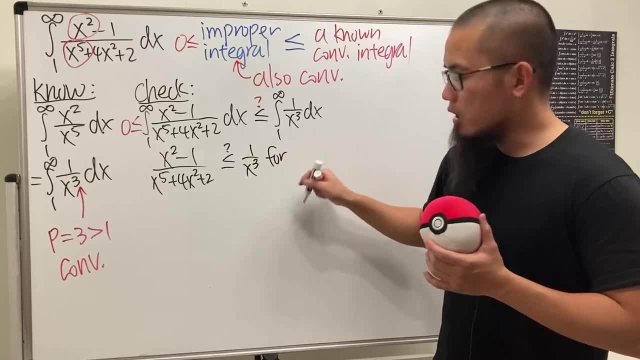 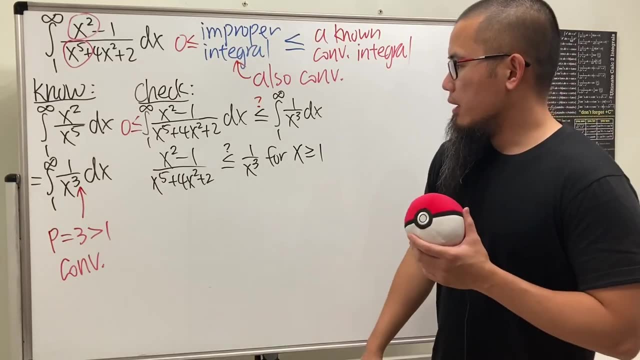 that which is one over x plus third power, and we just care about four x's, from 1 to infinity. so we just say: for x is greater than or equal to 1, okay, again, everything's positive when x is greater than or equal to 1. in fact, when x is 1, the left. 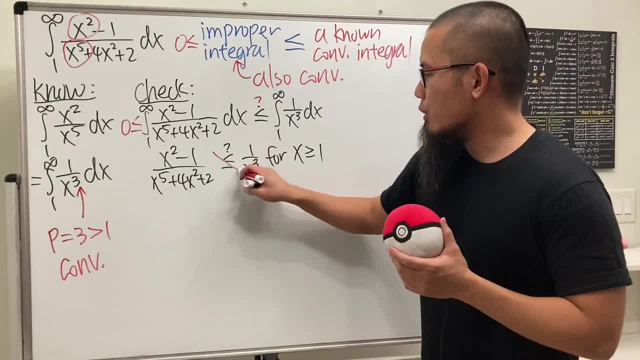 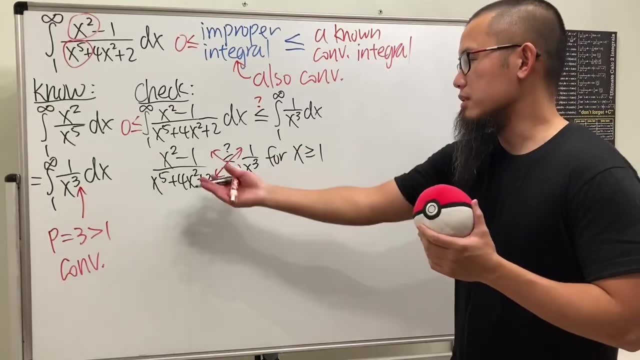 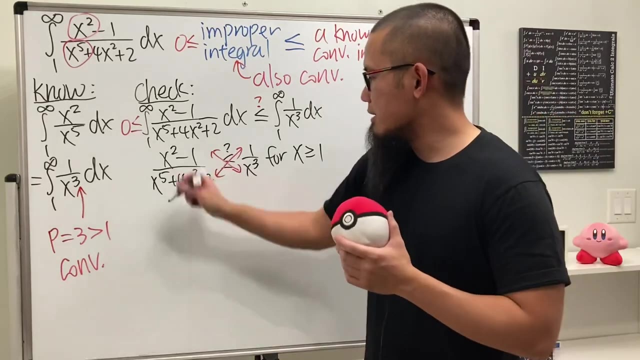 hand side is 0, but it doesn't really matter. we can still cross, multiply and we still keep the same inequality because it's not 0, because it's not negative, so we don't have to switch the inequality anyway. go ahead, multiply this and that which is x to the third power times: x squared. 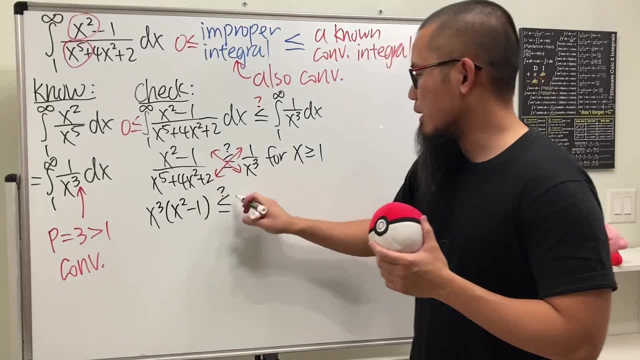 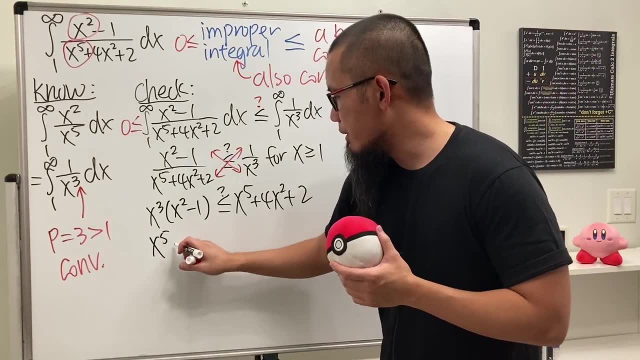 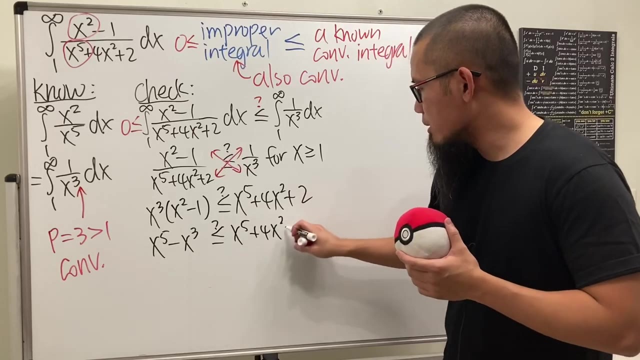 minus 1. is this less than or equal to, this times that which is x to the fifth plus 4x squared plus 2? work that out real quick: x to the fifth minus x to the third power. is this less than, or equal to, x to the fifth plus 4x squared plus 2? well, cancel, cancel, and we can move this to the other side. 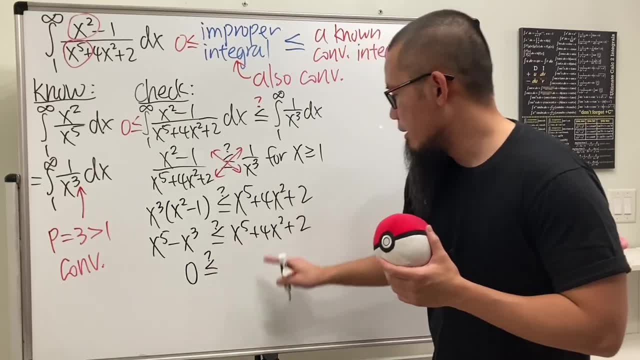 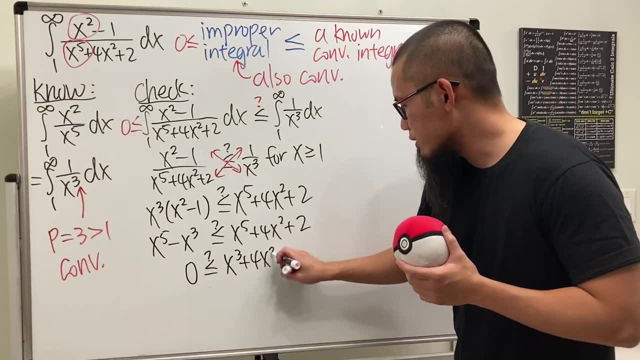 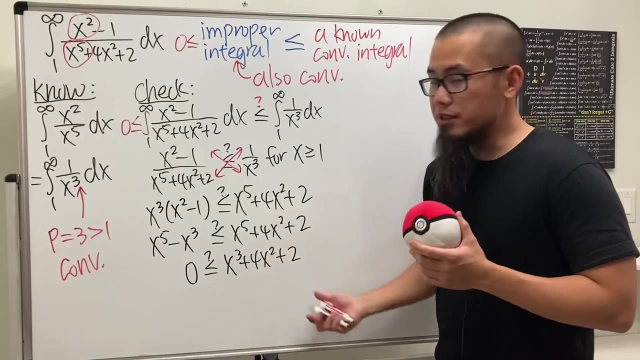 so we're looking at 0 less than or equal to- and i will write down x to the third power first, and that's positive. and then we have this 4x squared plus 2. well, check this out: when x is greater than or equal to 1, you know everything here is going to be positive, right? you're adding all the things. 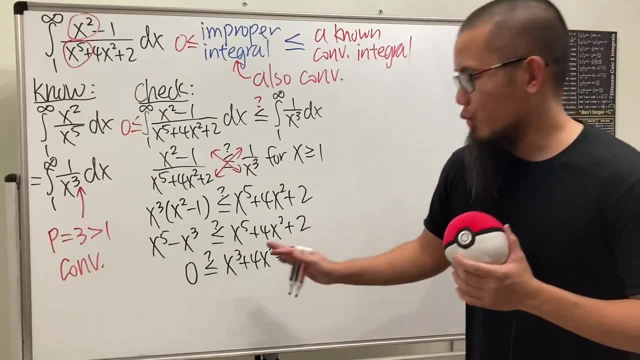 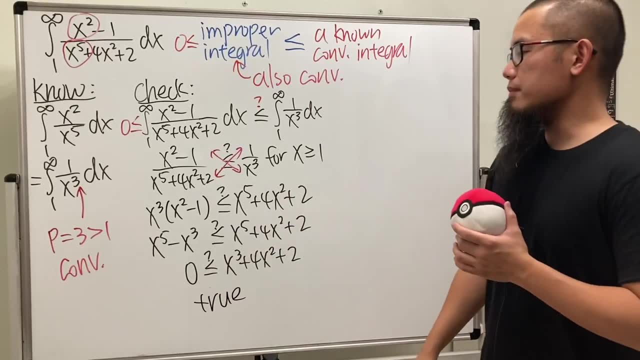 are positive. so you can be sure that this right here is so greater than 0 when you look at it backwards. so this right here should be super clear. that is true. yay, we can draw conclusion now. so we'll come here and then write down our conclusion. 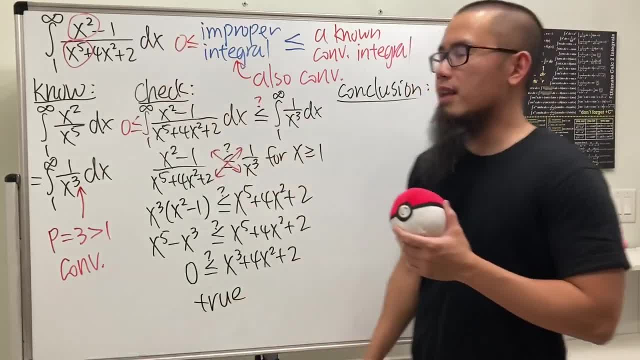 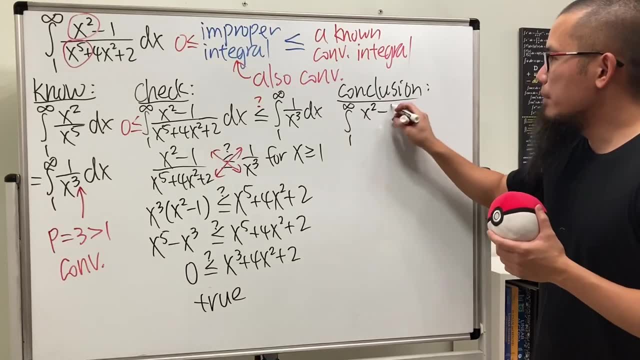 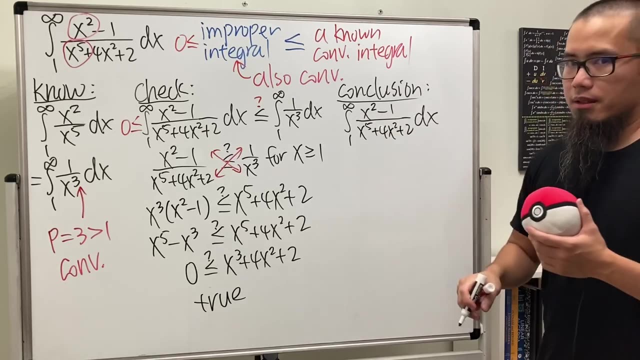 and again. the conclusion is that we are going to write down the original and we are going to make it clear, like: what's up with that? x squared minus 1, over x to the fifth, plus 4x squared plus 2. you know the magic work also. 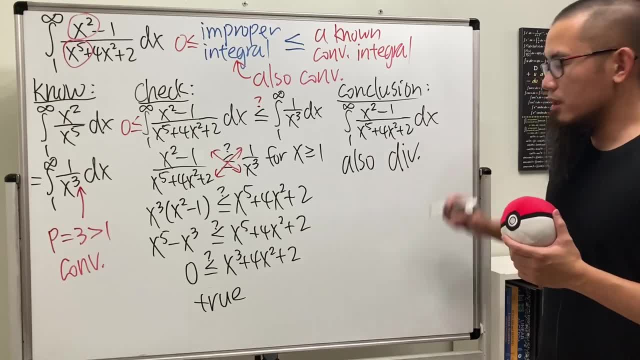 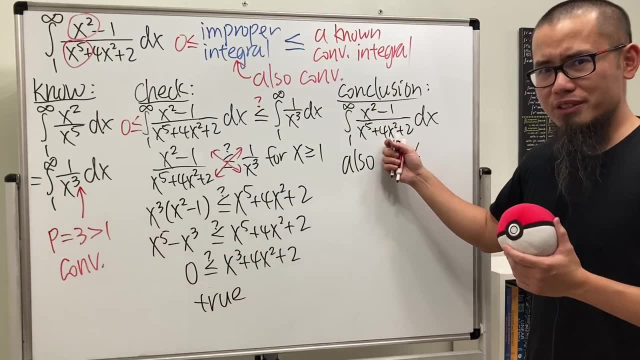 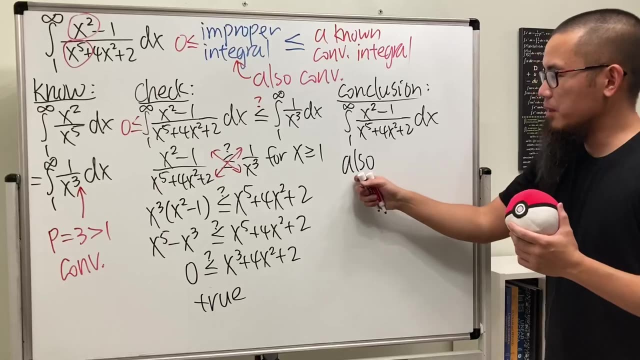 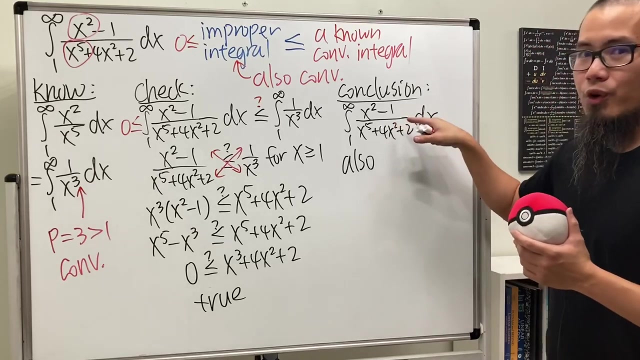 also what diverges. does this sound right? this right here converges. this integral right here also diverges. it doesn't sound right. well, this right here. is why that keep emphasizing using the word also because it will help you to write down the last statement correctly: this right here also. 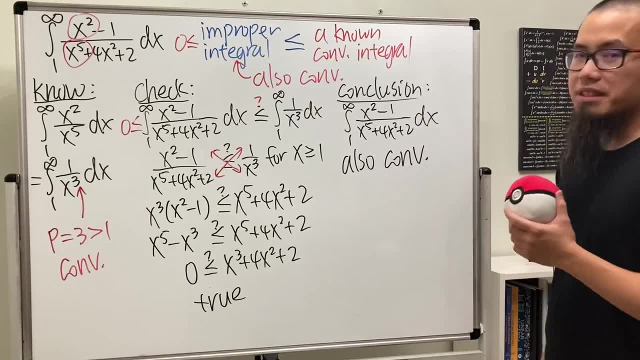 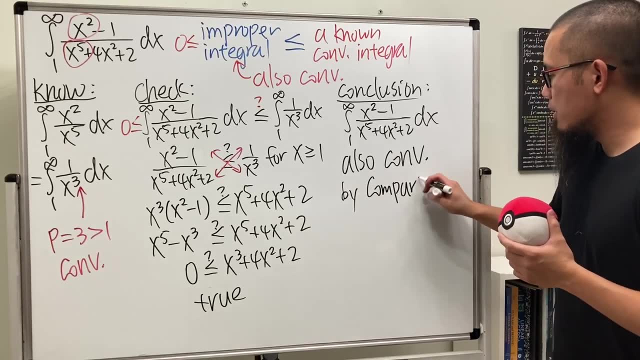 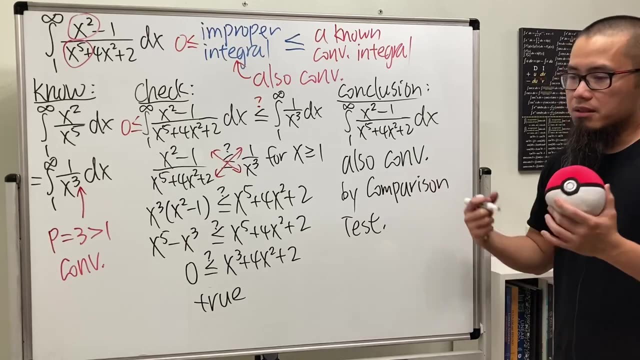 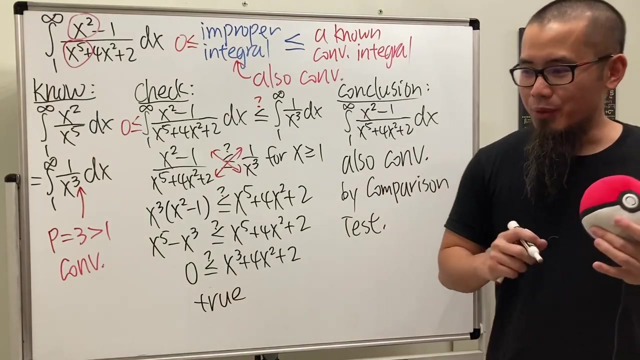 converges, all right, and then, of course, can also just quote the name of the test that we're using by the comparison test, and the reason that i just want to keep writing down like by the comparison test is that it's just a good habit, because we are going to be doing the infinite series pretty soon and for that we will have